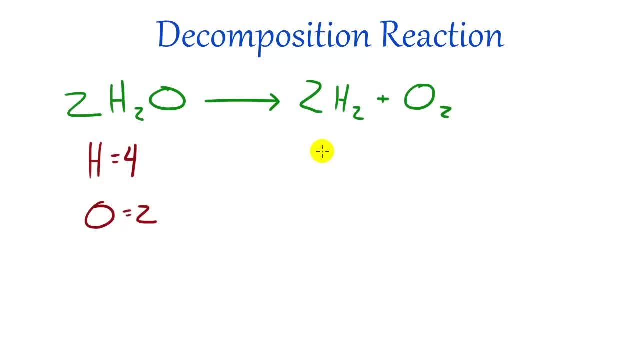 Now that's what we started with and we need to make sure we ended up with the same amount of stuff that we started with. So if we go ahead and look at this in H2, two hydrogens, So we have four hydrogens, since 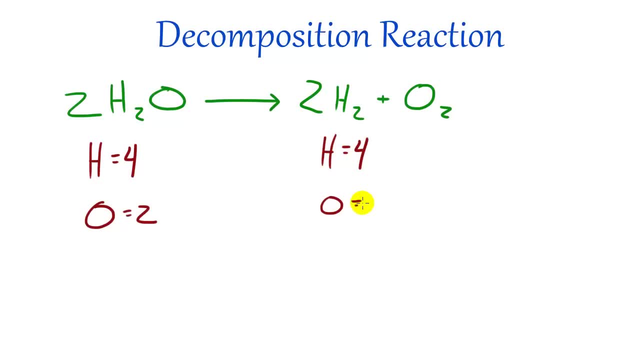 we have two of them, And also this one is simple. We have two oxygens, just like that. Simple enough. So now let's go ahead and look at another example before I give you guys your first assignment. Actually, I think I gave you guys an assignment before, But let's. 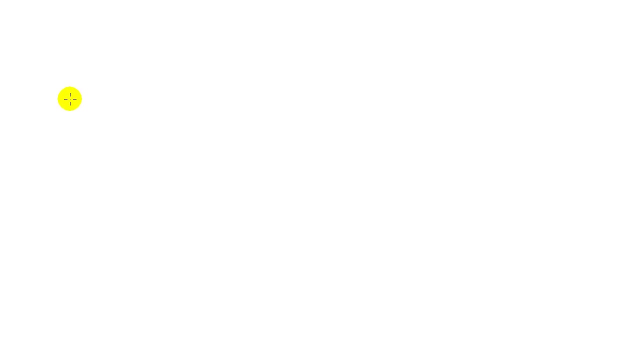 go ahead and take things up a notch and take a look at something called calcium carbonate. The formula, oh, that is quite embarrassing. The formula for calcium carbonate is CaCO3.. And I know, I don't know, never mind, I was just rambling, But anyways, what you do is. 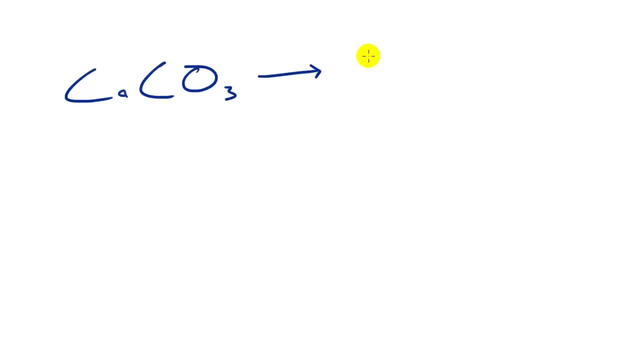 you take this calcium carbonate and split it up and you end up with CaO2 plus carbon dioxide, which is CO2.. Now let's go ahead and balance this bad boy. And again, remember, this is a decomposition reaction. You take one thing and you break it up into two or more things, just like that. So that's. 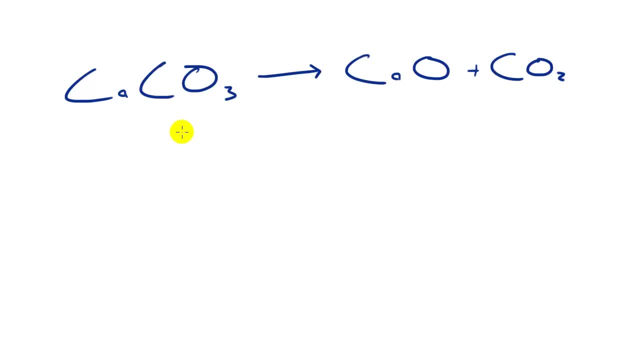 basically what I'm telling you guys how to do. So let's go ahead and balance this one more time, And you guys are going to want to pay attention because you guys have some homework to do coming up And you're going to need to balance some reactions. 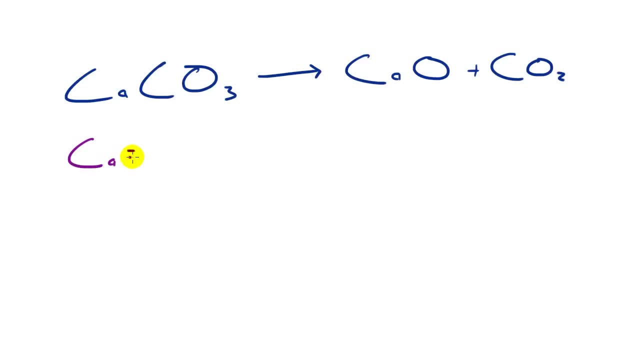 So we have one calcium, We have one carbon And we have three oxygens. Now let's go ahead and just cancel all this. So let's go ahead and cancel this out. Calcium: we have one, So let's go ahead and cancel that out. 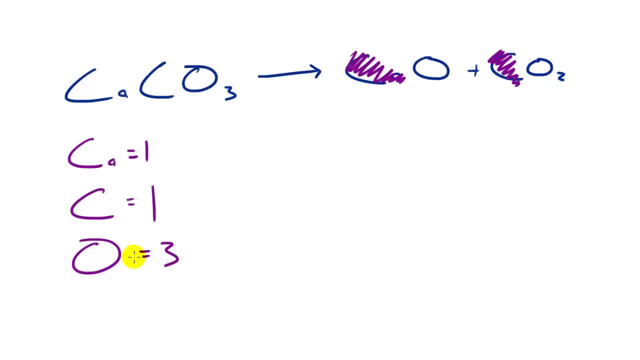 For carbon we have one, Here's one, And for oxygen we need to find three. Here's two, And here's another one. three, And as long as you cancel everything out, everything is out and nothing is left over, then we're good to go. 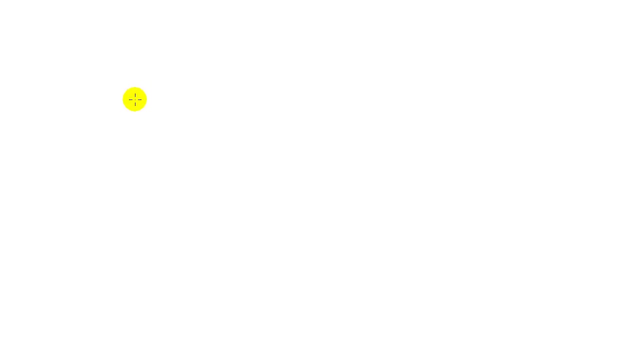 So here is your homework assignment for the evening. What you're going to do is you're going to find out how many molecules of oxygen are left in my potassium chloride. Sounds fun, So we're going to go ahead. and OK, that's getting annoying, We're going to go ahead.